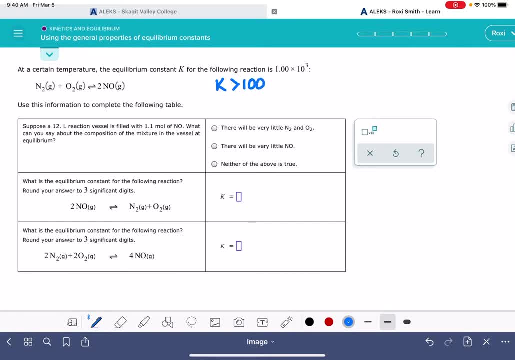 constant is large, and by that we define is being something greater than 100, that means that we have in our system more products than reactants. This equilibrium constant is large. It is greater than 100.. That means that we have more products than reactants. So that means we have more NO than N2 or O2.. 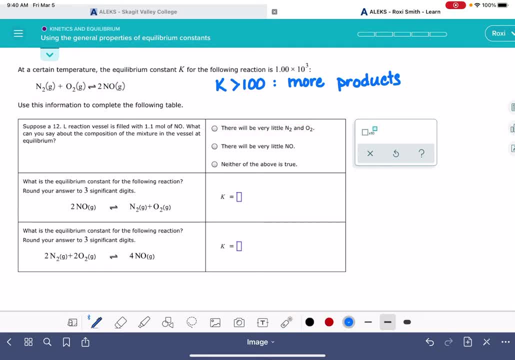 So the way that this, the answer that we would select, that would be the most appropriate. there would be very little N2 and O2.. It's going to be NO Now, even though it doesn't apply to this problem, if your value of k is. 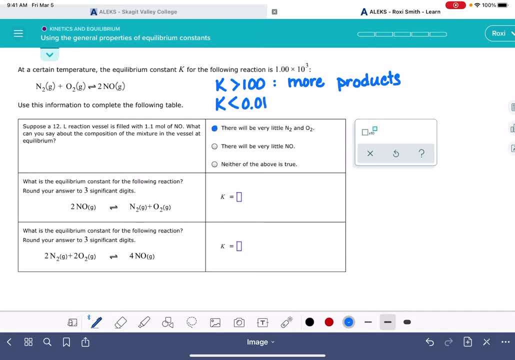 small, and we define that as being less than 0.01,. in that situation you would have more reactants than products. And if your value of k is somewhere in the middle- so somewhere between 0.01 and 100,, then we say we have a pretty even balance of reactants and products. 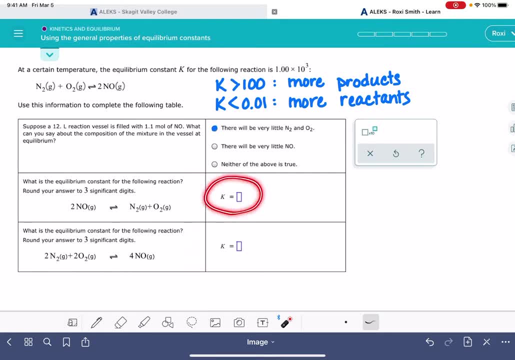 The next two questions, it will ask you to calculate a value of k. So if your value of k is for a slightly different chemical reaction, it's going to have the exact same molecules. They're just either not going to be in the same order or their stoichiometric coefficients will. 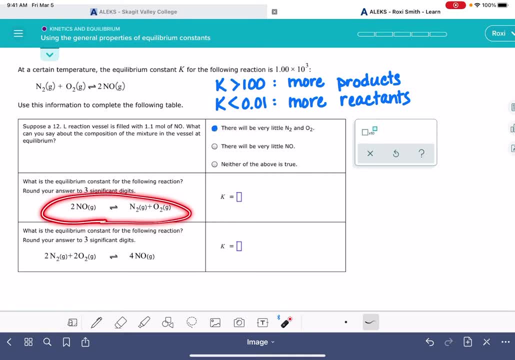 have changed In this particular one right here. when we compare this equation to the provided equation, we can see that it's just been turned around. So the reactants are being written as products and the products are being written as reactants. When an equation is turned around, 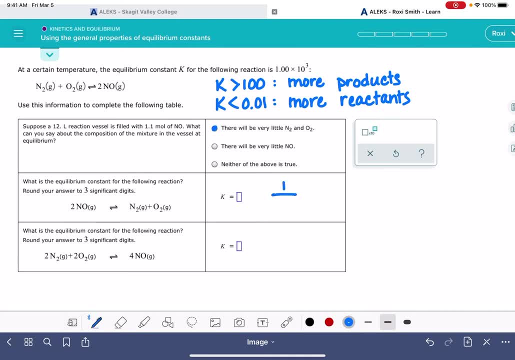 then the value of k is inverted. So if k is 1 times 10 to the 3, then when we turn the reaction around, k is going to be 1 over 1 times. why did I write 10 to the 1 times 10 to the 3.. So when we turn the reaction around, we invert the value of k. 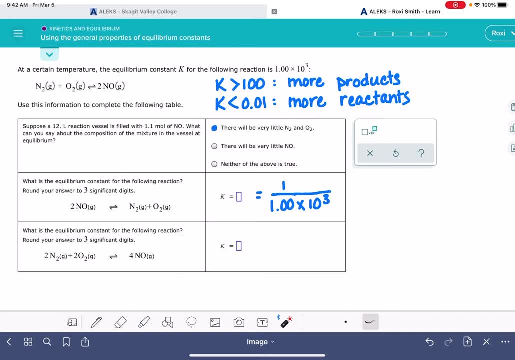 Don't enter it into Alex like this. We want to enter it in as 0.001, or 1 times 10 to the minus 3.. And in this second one I have here, I'm going to write 10 to the minus 3, and I'm going to write 10 to the minus 3.. 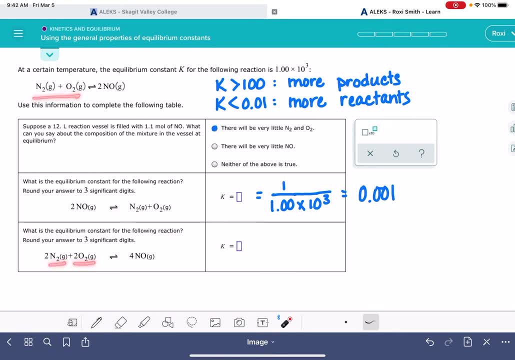 And here I have: my reactants have not been moved. So my reactants are still reactants and my products are still products, But the stoichiometric coefficient has changed. The stoichiometric coefficient has doubled. So when you make a change to the stoichiometric coefficient,